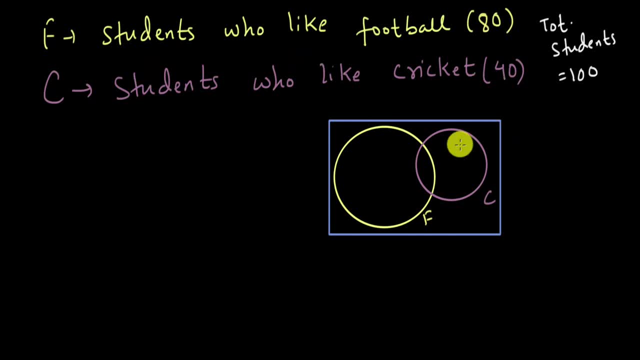 ki 80 students hai who like football and 40 students hai who like cricket. and there are some students jo ki yaar pe hungi jinko dono pasand hoga, football bhi, cricket bhi. alright to, let's say ki yeh jo students. 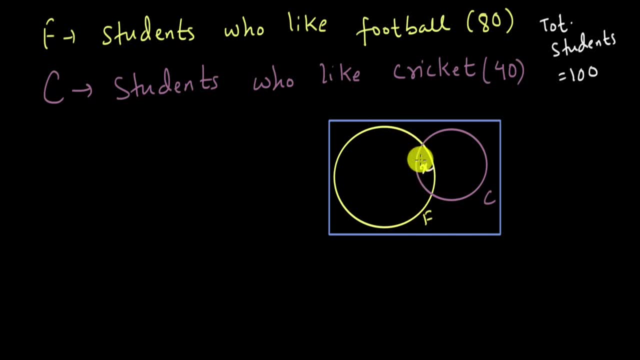 jo yaar pe hai. they are X in number to agar X students aise hai out of 80 jinko football aur cricket dono pasand hai. to aise kitne students hai jinko sirf football pasand hoga. 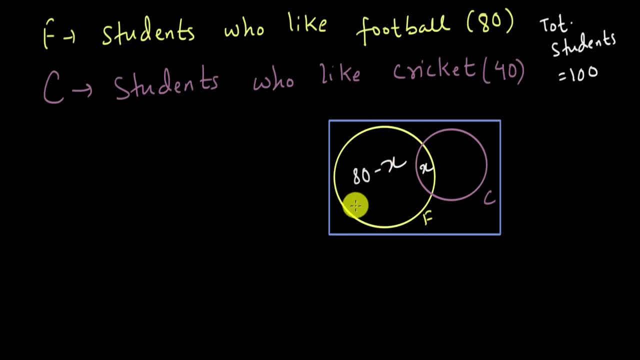 wo hongi 80 minus X hai ki ni 80 students total hai jinko football pasand hai, unme se X aise jinko cricket bhi pasand hai. so 80 minus X is the number of students who like. 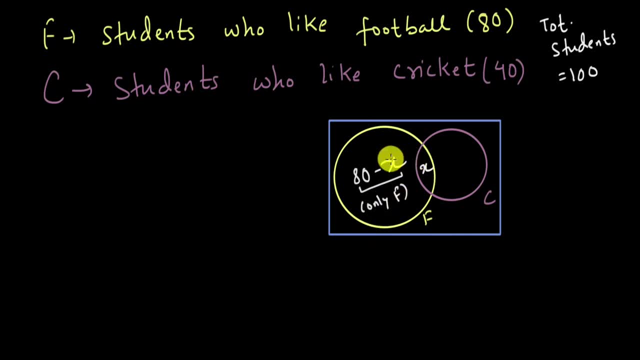 only football correct. similarly, agar mai aapse puchu ki, agar X students aise hai, jinko football aur cricket dono pasand hai, aur 40 to total students hai jinko cricket pasand hai to aise kitne students honge jinko. 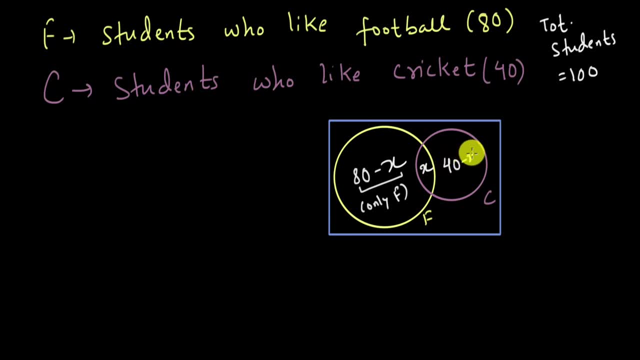 sirf cricket pasand hoga. waise students bhi hongi 40 minus X inko sirf cricket pasand hai only C. yes, alright to ab agar mai in 3 no portions ko 80 minus X, jo ki mera only F wala portion hai. 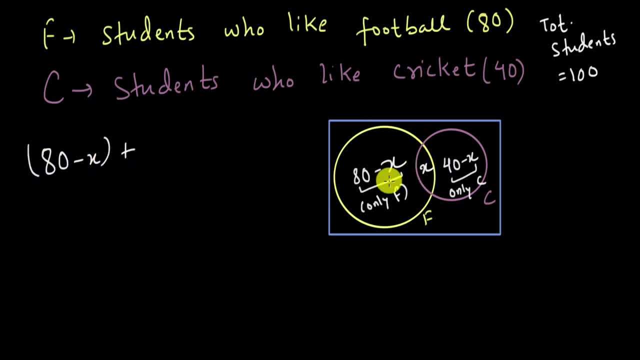 usko plus common portions: jo ki mera X hai plus 40 minus X, jo ki sirf cricket wala portion hai, only that is cricket portion hai. inko add karu to ye addition: iska sum kiske barabar ho na chahiye This. 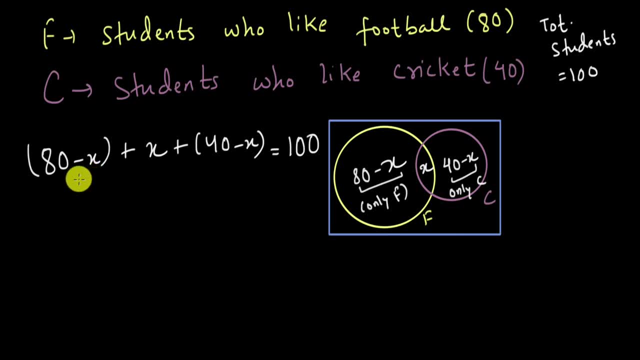 should be equal to 100.. 80-x students aise hai jinko sirf football pasand hai, x aise jinko dono pasand hai, aur 40-x aise jinko sirf cricket pasand hai To football ho gaya. 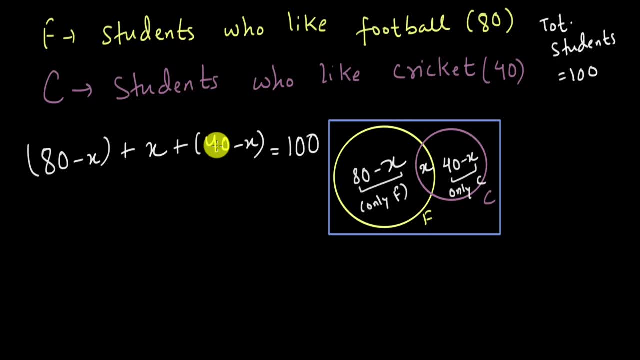 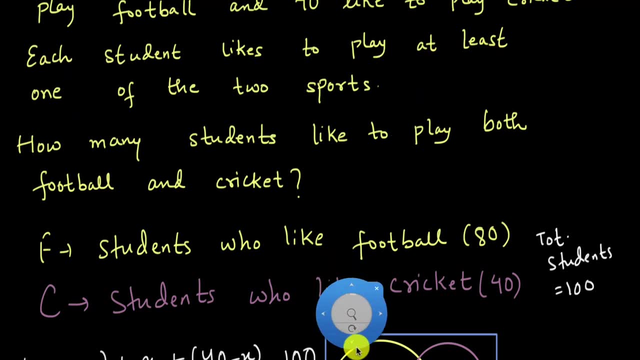 cricket ho gaya aur dono wale bhi ho gaya. To now we have covered all the types of students. Aapko yaad hai question me given tha that each student likes to play at least one of the two sports. To aisa koi bhi nahi hai. is class mein jisko koi sport khelna pasand? 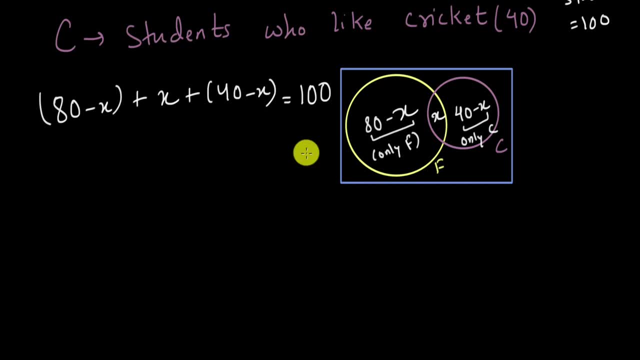 nahi hai na football, na cricket, Yaani in tino groups ko mila, ke humne saare students cover kar liye hain. To the total is 100.. Ab ma eger isko solve karu, then I'll get. 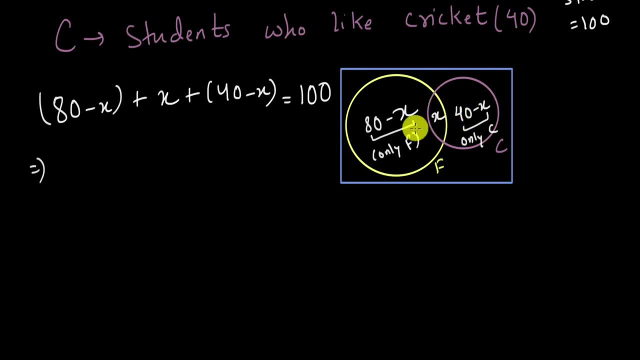 my answer of how many students like playing both football and cricket. So this gives me 80 plus 40 is 120, minus x plus x cancels this gives me 120, minus x is equal to 100, and this means 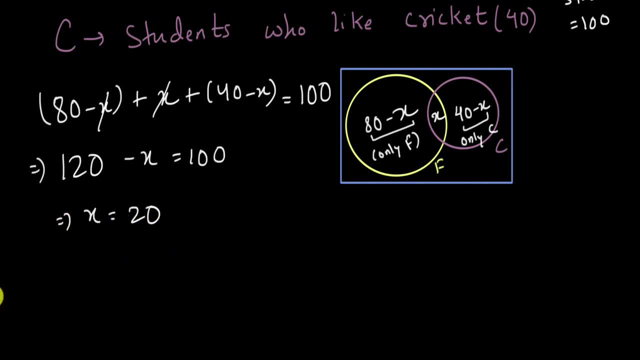 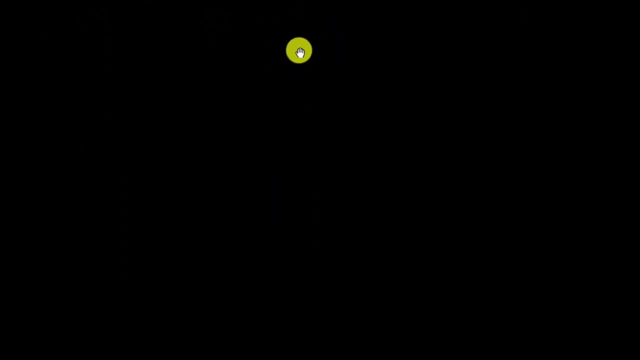 x is equal to 20.. So this is the number of students who like to play both football and cricket. To ye to humne iss case mein solve kar liya. But yahaan pe hum ek general pattern bhi dekhne ko mil raha hai, jisse hum ek property derive kar sakte hain. Dekhte hain in general. 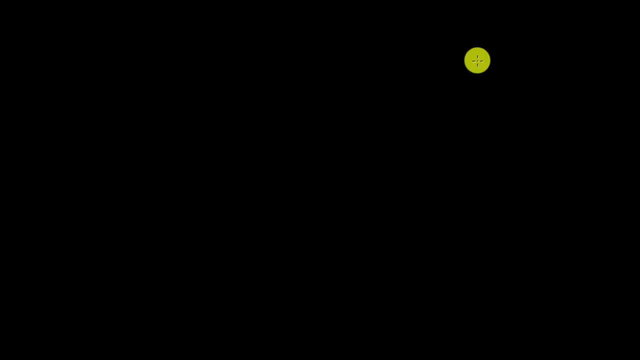 agar mere paas 2 sets hoon, phir se 2 sets banate hain, A and B, to in general ek relation derive karne ki liye main yahaan pe in 3 areas ko phir se add karta hoon. 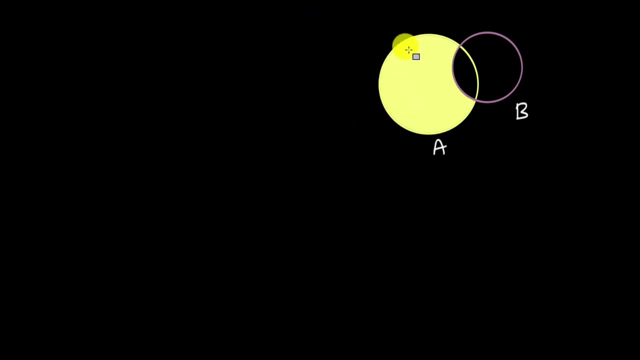 Pehla area hai mera ye doosra area hai mera ye, aur teesra area, jo ki dono ke liye common hai. woh hai ye In 3 areas, ko mai add karta hoon, So A, the area. A is basically the total. 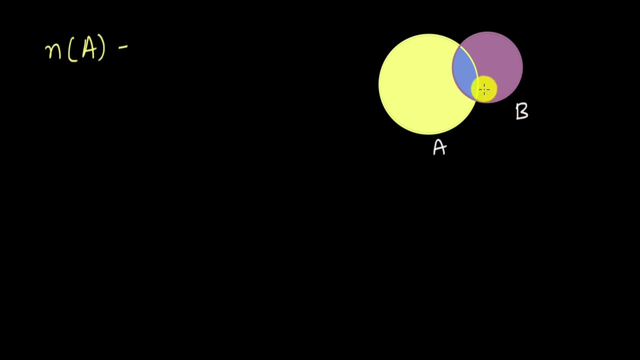 number of elements of A, minus the elements which are common, yani minus the elements which are in the intersection of A and B, Kya mai ye likh sakta hoon. This is the yellow portion, Correct, Plus plus blue portion. mein humare paas sirf intersection wale elements hain. 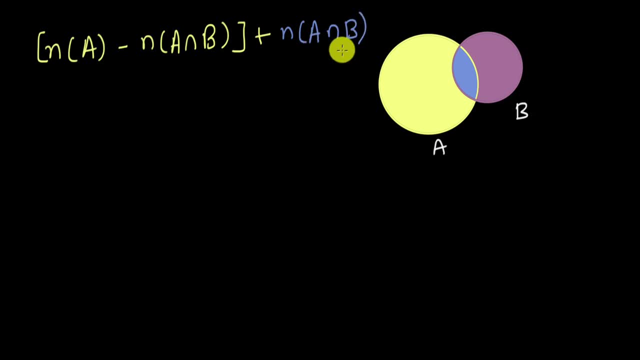 yani number of elements that are both in A and in B, And then again plus we are adding this area, the purple area. this has the number of elements of B, minus again, common area, Pure B. mein se maini ye blue area hata diya yani minus N of A, intersection B. So this: 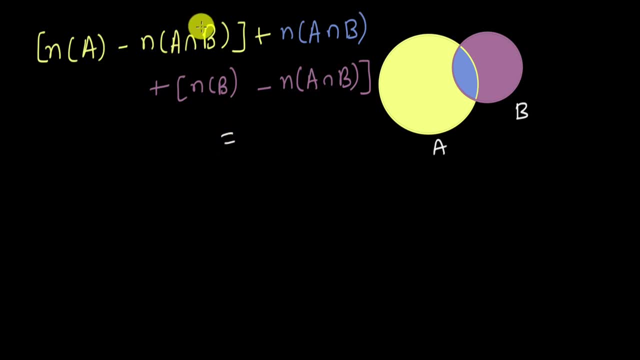 is my purple area To ab agar iska mai total karu to merko dikh raha hai again wahi cheez jaise. minus x plus x, cancel ho tha ye, cancel ho gaye. And this gives me N of A plus N of B minus N of A intersection. 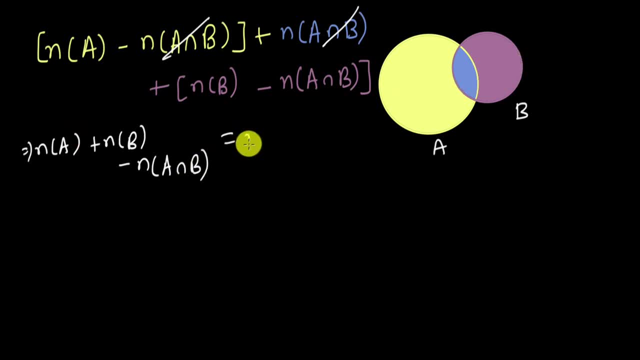 B, And this thing is equal to the number of elements of the union In 3o ko combine. karte hain to isko hum kya bolte hain Isko union bolte hain To ye mera ek relation hai choki.